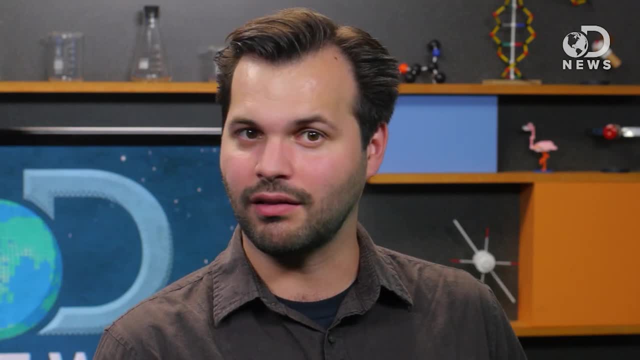 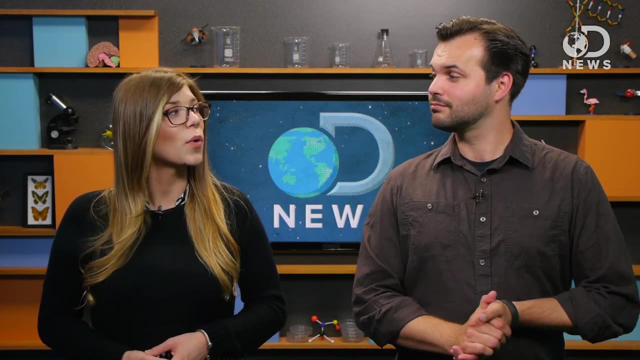 the proteins in the meat to coagulate, transforming it into a milky white color. And that same process occurs in every kind of animal, Which is why raw meat always looks different than cooked meat. So what about salmon? the oompa-loompas of the sea, Which is a new name I just gave them. 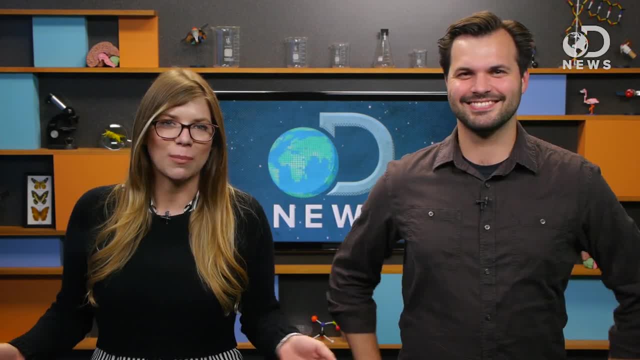 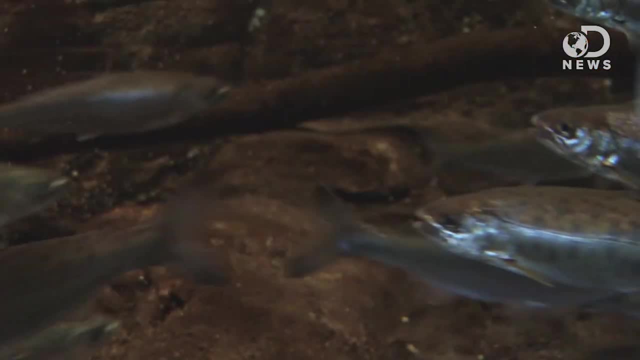 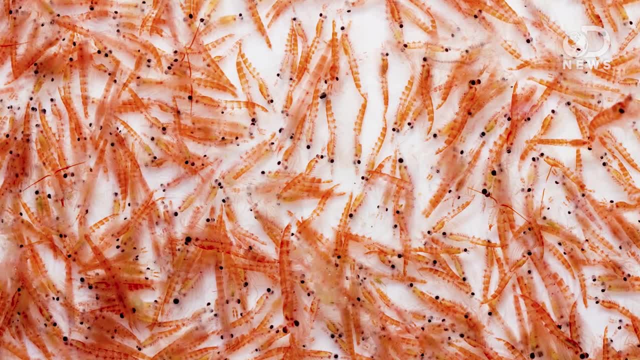 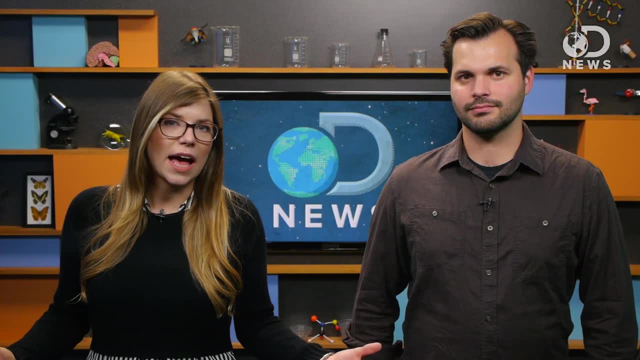 are really fond of eating krill And krill are really fond of eating algae, And the algae they eat contains carotenoids, which are pigments that give food and plants their bright colors. So when krill eat algae and salmon eat krill, the salmon is indirectly 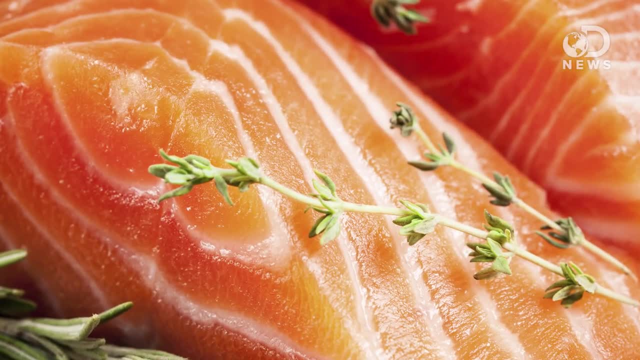 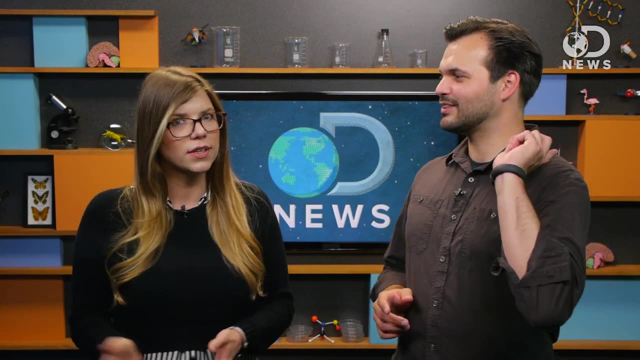 consuming those carotenoids which in turn gives their flesh a bright orange color. But salmon aren't the only fish who eat krill, So why are they orange and the others aren't? That is where the genetics part comes in in. Most salmon have a color gene that allows carotenoids to penetrate their muscle tissue. Some salmon, however, lack that gene, so, even though they're identical to the orange salmon in pretty much every other way, their flesh is a grayish white color. 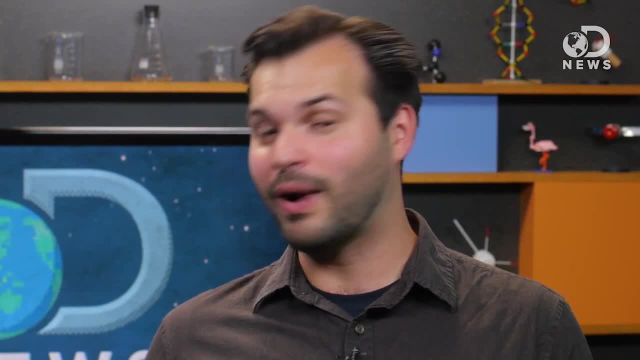 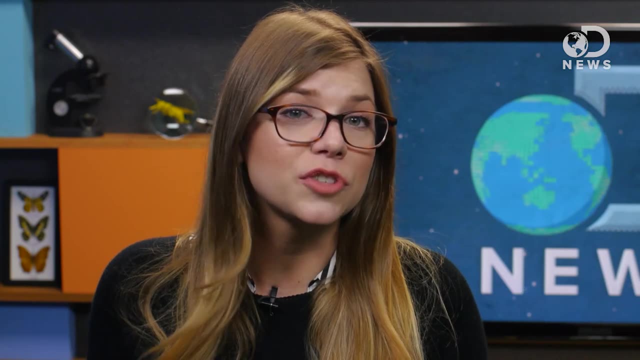 They're called ivory kings and typically they sell for a bit more than regular salmon, Though they can be hard to get off the shelves because people are so used to seeing that orange color. White fish need love too, as do blue fish, the jewels of the sea. 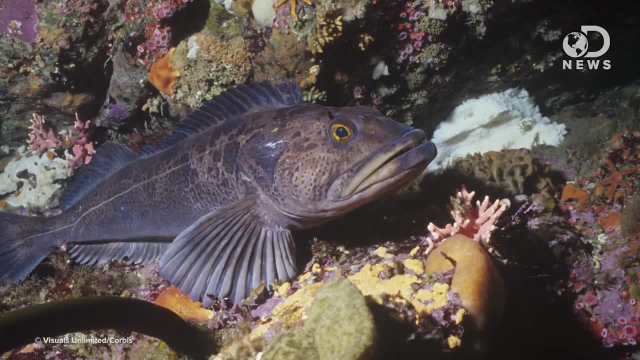 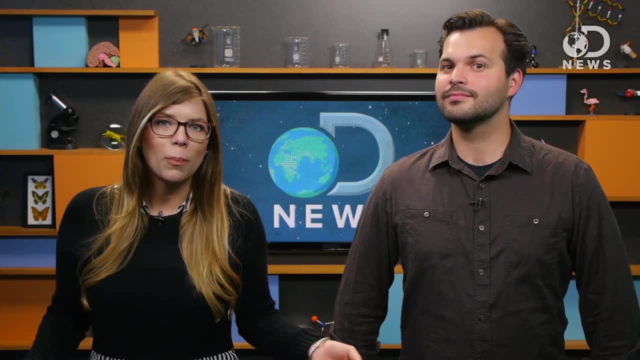 Another great nickname given by me: The blue lingcod. despite its name, is actually a white fish, just like halibut, but sometimes their flesh will take on a blue color And that's caused by a bile pigment called biliverdin which gets into the blood serum. 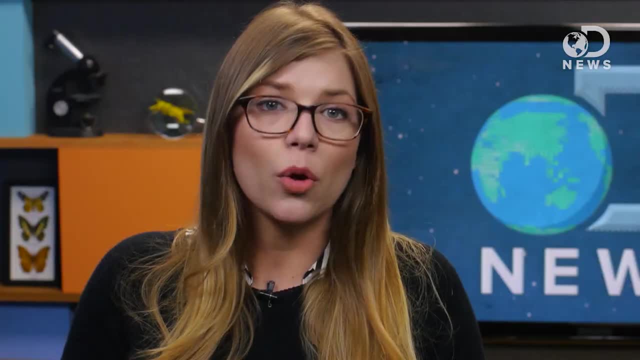 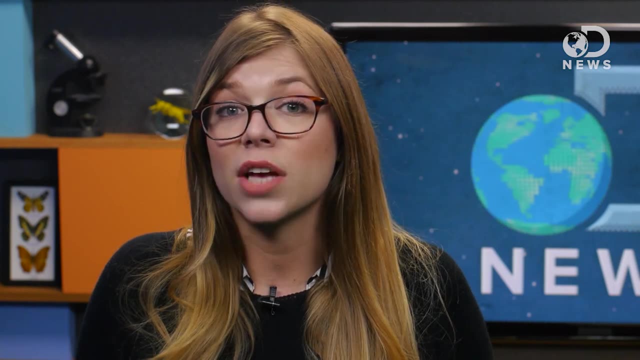 and turns their flesh into an extremely bright shade of blue. The question of why this only happens to some fish, or any fish at all, is a complete mystery to biologists. But it's definitely not relegated to just lingcod. The rock greenling and the kelp greenling, which are both cousins to the lingcod, have 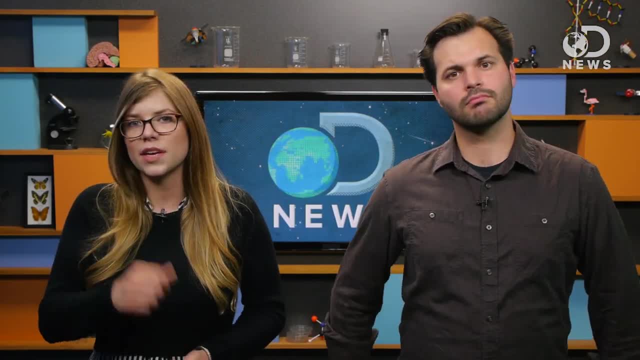 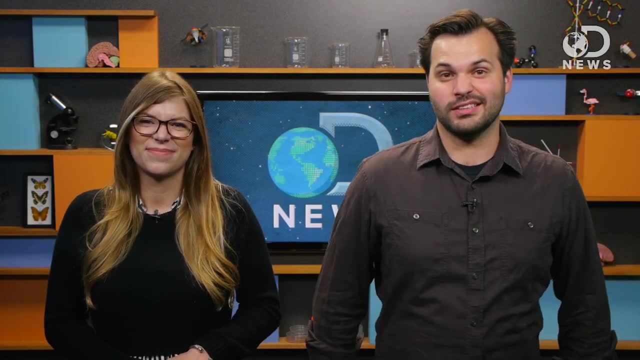 also been known to have the same color. They're known to adopt a distinctive turquoise color, though that's a pretty rare occurrence. Personally, I can't imagine eating a turquoise fish, but apparently they taste the same as the white ones And once you cook them their flesh turns back to white anyway. 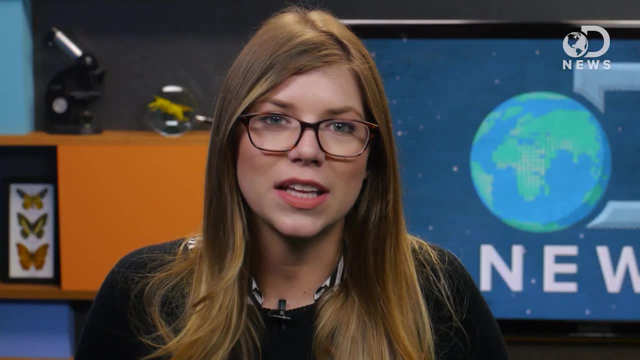 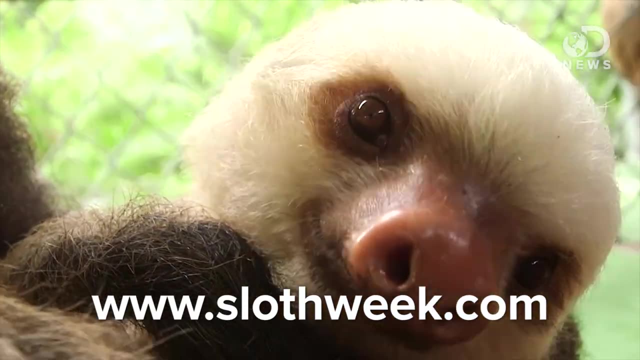 Animals are amazing Totally. While we're on the subject of animals, let us remind you that it is currently sloth week here at Discovery, so all week long we're going to be uploading adorable sloth-related videos for you to quad over. 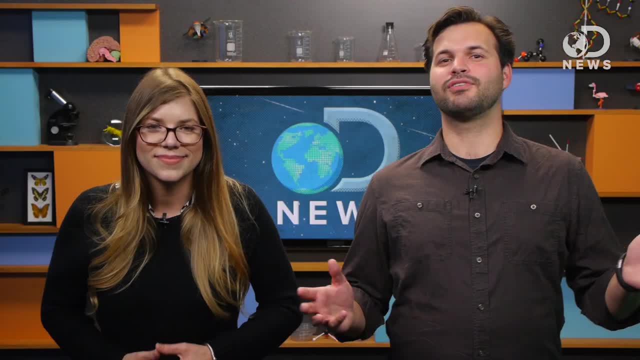 If you want to see all of them, just head over to slothweekcom. In the meantime, if you have questions, comments or favorite topics, let us know in the comments If you have a favorite type of sushi you want to share with us, just leave it down. in the comments. Otherwise, thanks for watching. 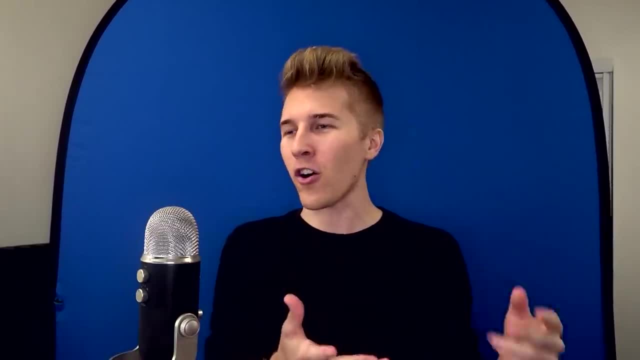 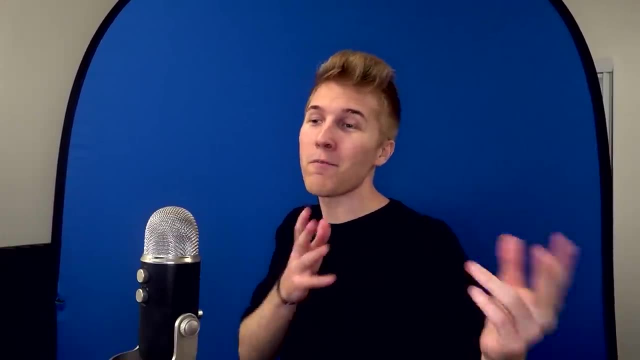 I've done one tier list video and it was kind of a joke. I was ranking all countries of the world and I didn't want to take it too seriously- People still, of course, did- and I made a lot of people mad, and I'll make a lot of people mad today, Maybe even more mad because I'm going to take this. 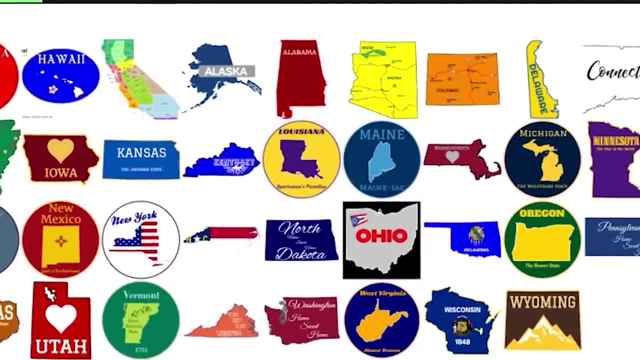 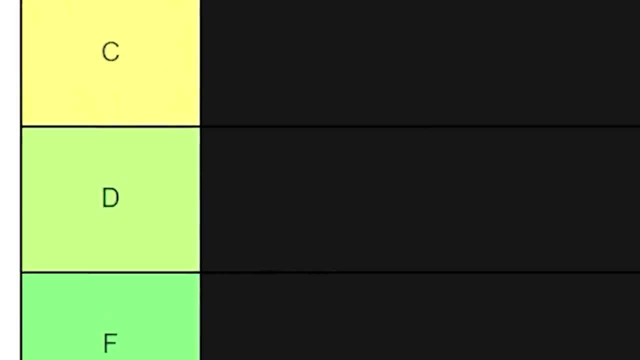 a little bit more seriously. I've done a lot of like games where we have a battle royale take place between all 50 states, Just basically a huge free-for-all, big old conflict. I want to like seriously ask myself who I think would do the best and I'm sorry in advance, when I'm going to 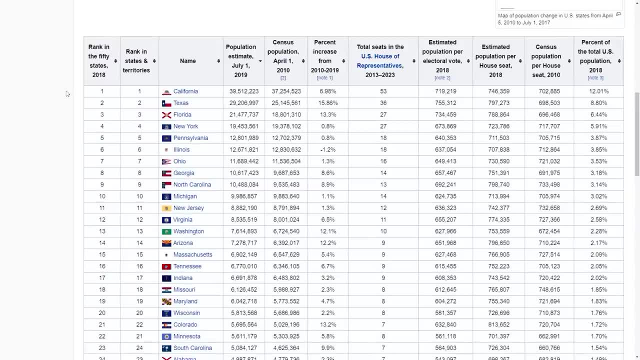 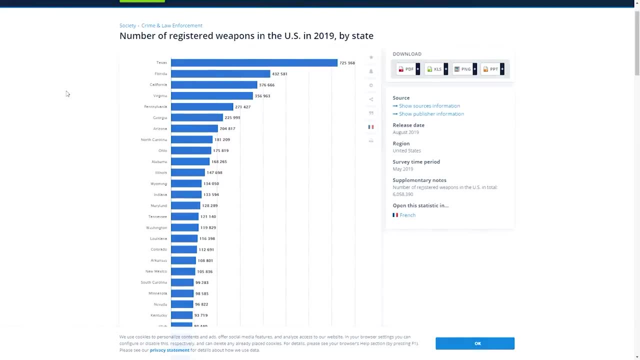 make a lot of people mad. It's just my opinion. It's just my opinion. Now I'm gonna look at some data, I'm gonna look at some information to assess my opinion and that way I'm not just like throwing things out there. All this stuff, I think kind of matters, Kind of matters to me. but uh, of course, 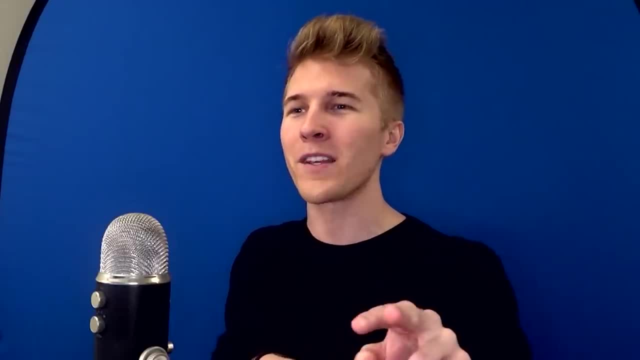 this is just my opinion. Let me know down below how wrong I am. Give me your top three. Give me your top three in the comment section Who you think would do the best, like the best in a battle royale. All right, I'm just gonna get this out of the way because everyone, and their mama is gonna. 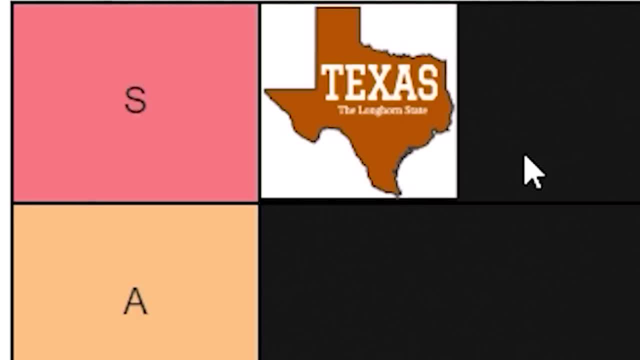 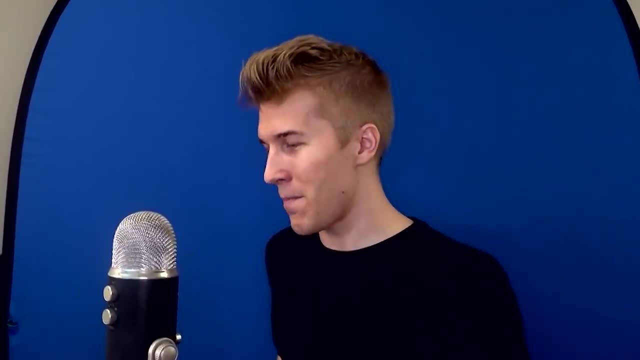 do this. Yeah, I think Texas would definitely be up there. You. just you gotta do it. I mean, they've already battled for their freedom once They still got the Alamo, Even though I don't think they're gonna be defending much in this sort of big old uh fight. 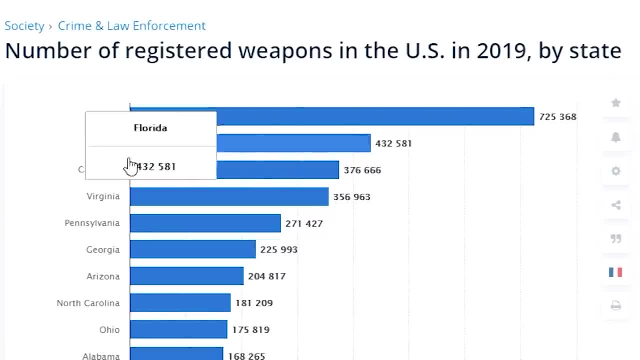 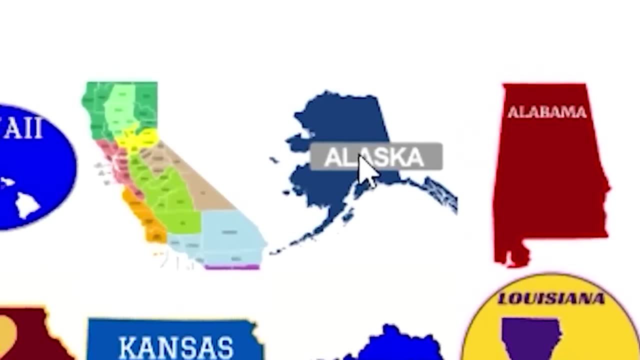 I think they'd be going out and expanding Also this, Also this. I mean, you know that that that helps They. they do have a lot of those, so, and a lot of population. Now, this one might be a little bit of a surprise to some people, but I'm actually going to do it. Alaska and uh, where are they?